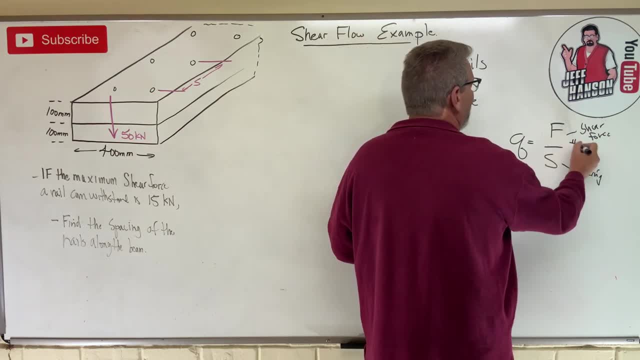 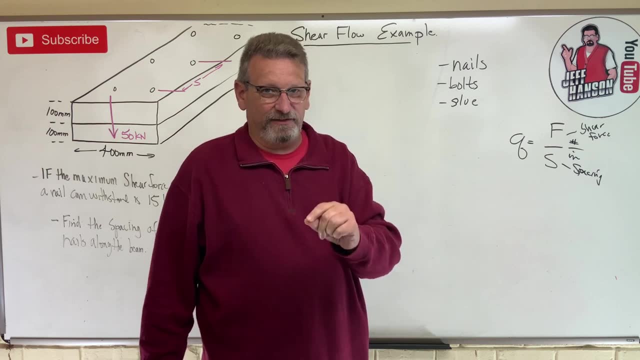 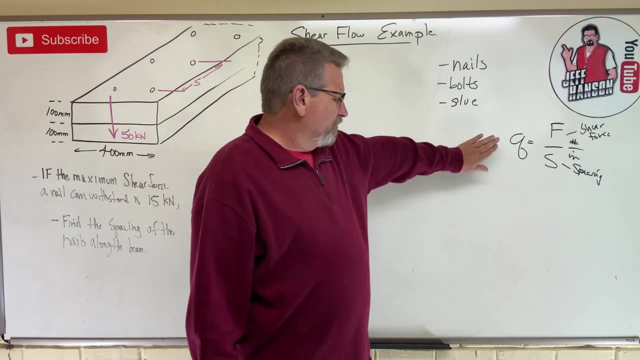 So this would be in shear force would be in something like pounds, and spacing would be in something like inches. okay, So the units are going to be a force over length every time, So Newton's per millimeter or pounds per inch, or whatever you got there, okay? So q equals force. 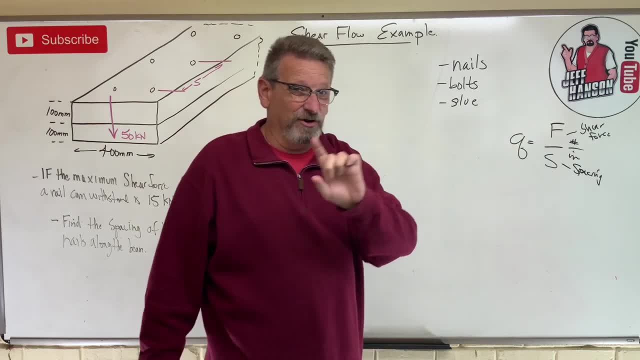 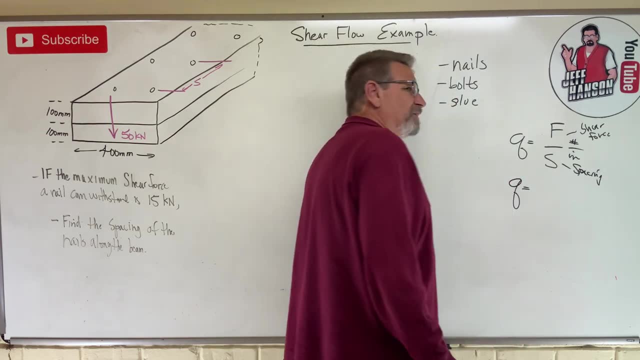 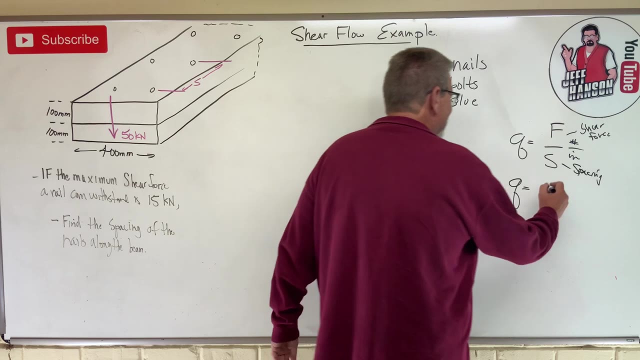 shear force divided by the spacing. Now there's another equation. My students call it the Vicky equation. okay, So if your name is Victoria or you go by Vicky, your street name could be little q. Okay, sorry, I don't know what just happened right there. okay, Vq over, i the Vicky. 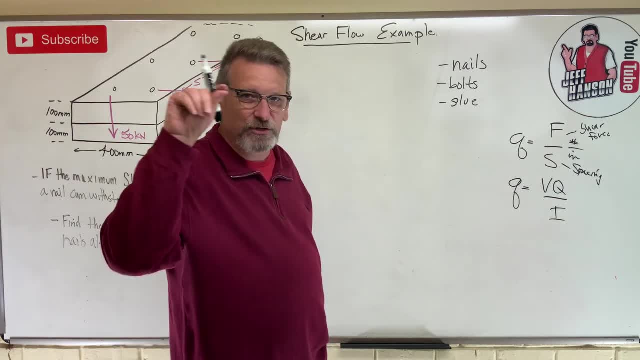 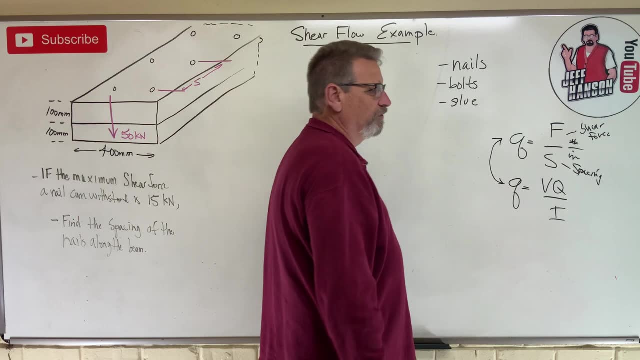 equation, not the Vicket equation. That was what we did. tau equals vq over it, if you remember, But this is another thing here. So this guy, this little q, is equal to that one, and this is shear flow. This is a way to calculate the distance between fasteners, okay, So let's see how this. 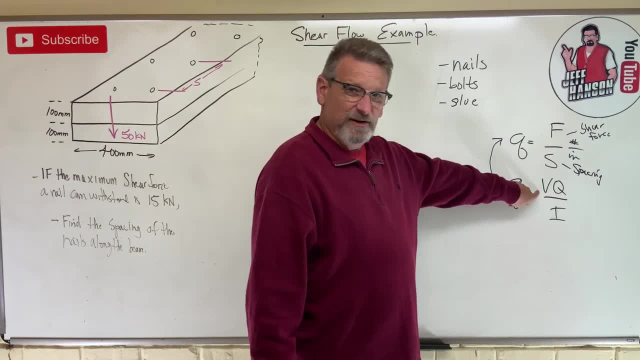 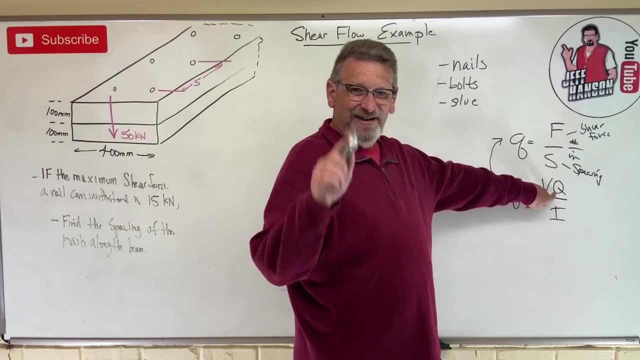 works. okay, We know what all the things are. We know the v is, that's shear force. Where are we going to find that In our shear moment diagram? yes, q, what is that? First area moment of inertia. 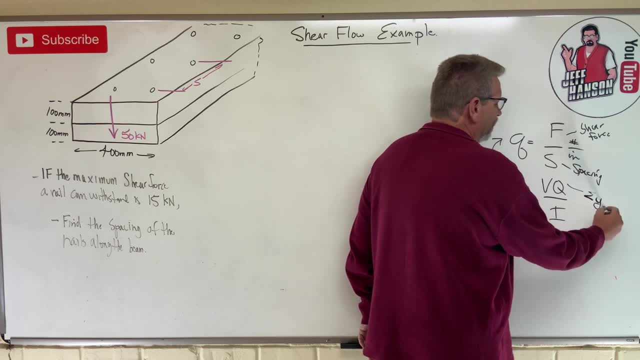 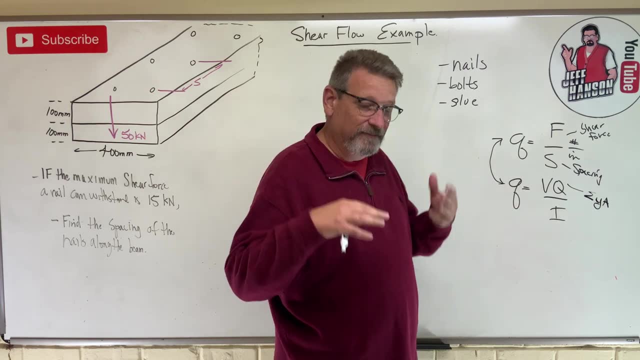 that is what The sum of the yas. remember that. And then i, the second area, moment of inertia. for rectangular beams, 1, 12th bh cubed. okay, So we know all the things in these equations. Let's see. 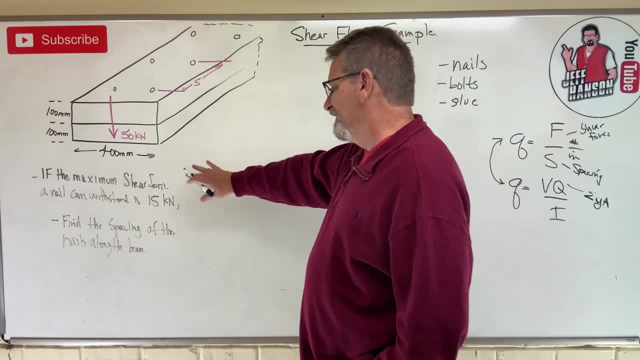 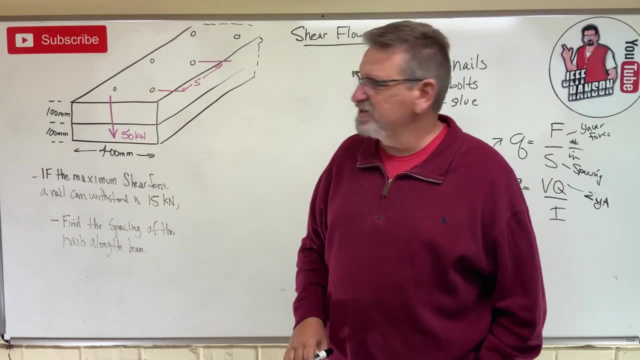 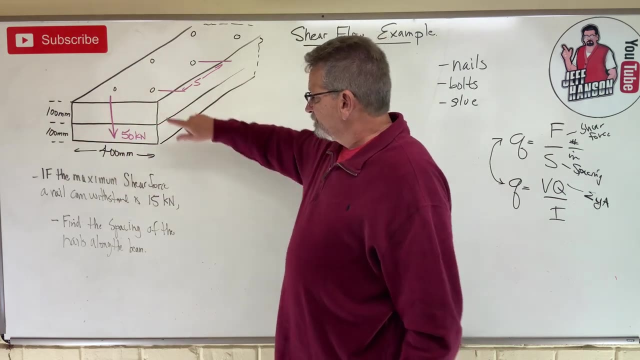 how we use them. okay, So if the maximum shear force a nail can withstand is 15 kilonewtons, what is the spacing of the nails along this beam? okay, So we've got two planks of wood that's 400 by 100, and they're nailed together ever so often. Now, how long is it? I don't know, It could. 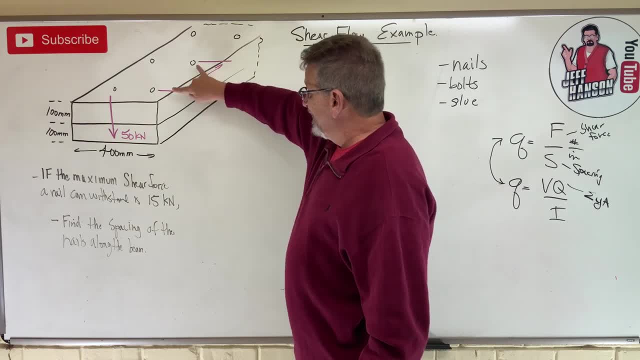 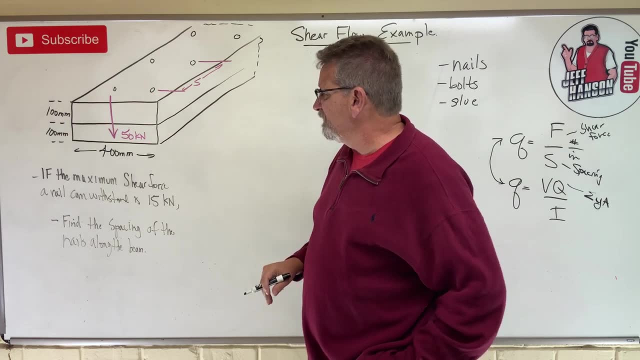 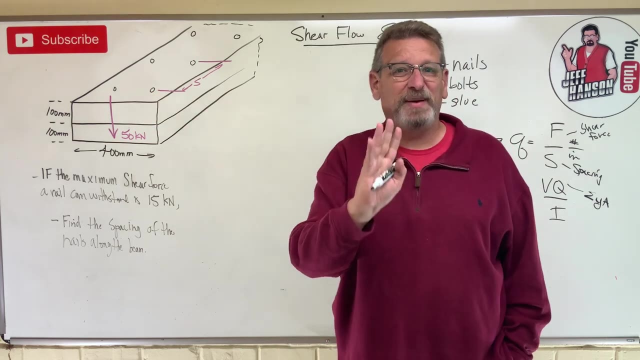 be forever long, I don't know, But what is the spacing that I need between the nails? okay, So let's see if we can do this. Now, one of the things that you have to understand on this problem is that these nails don't come one at a time. They come in pairs. okay, So if it's going to take 15, 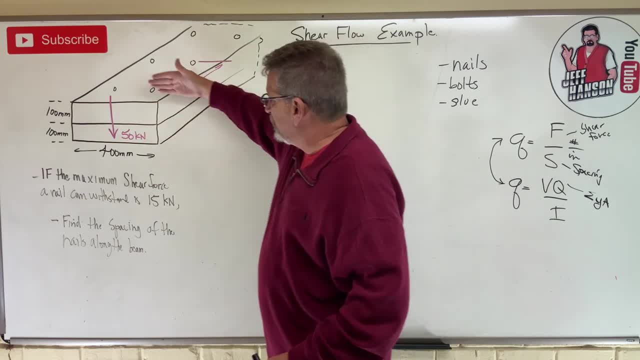 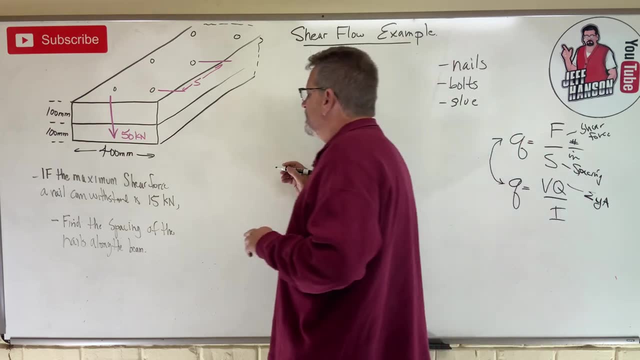 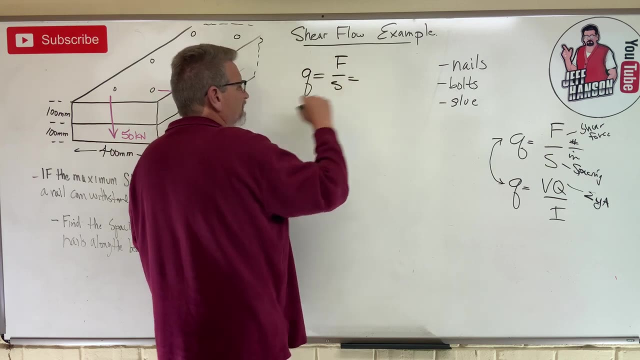 to shear that nail off, then to shear that row of nails takes how much? 30, right, I'm going to have to multiply by two, okay? So on this problem, little q is equal to f divided by s, which is: 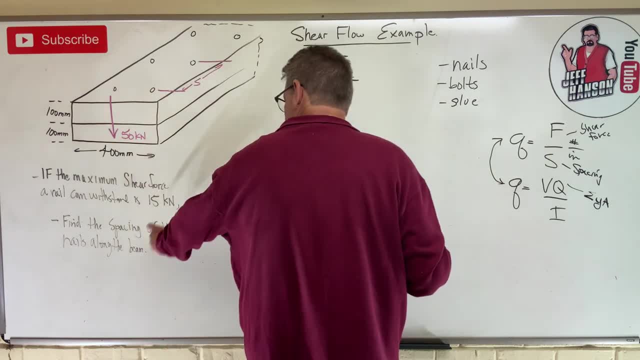 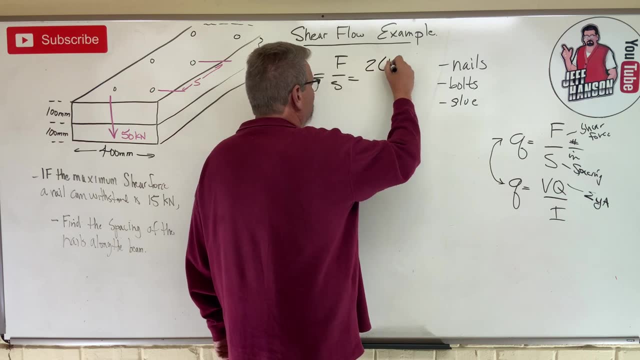 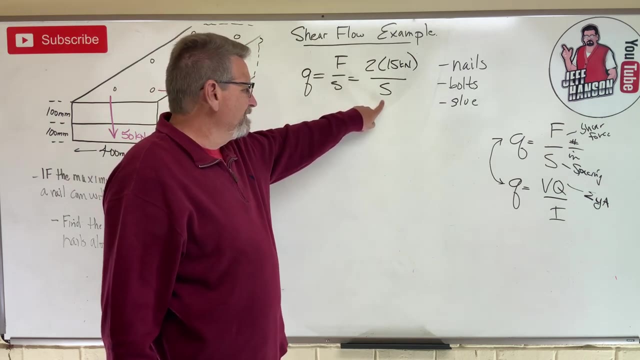 the force that it takes to shear a nail is given right 15 kilonewtons, but I got to shear two of them, So two times 15 kilonewtons. And then s that's what we're looking for, okay, Now what is q? I don't know, But maybe we can. 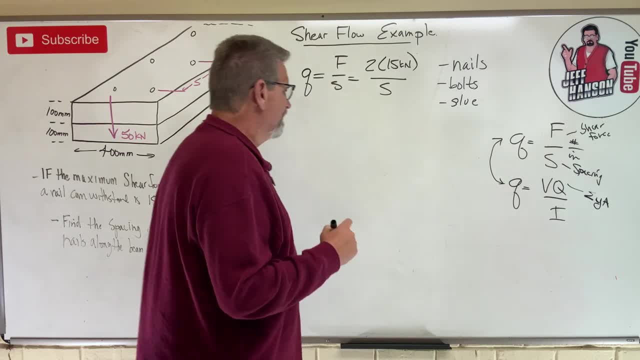 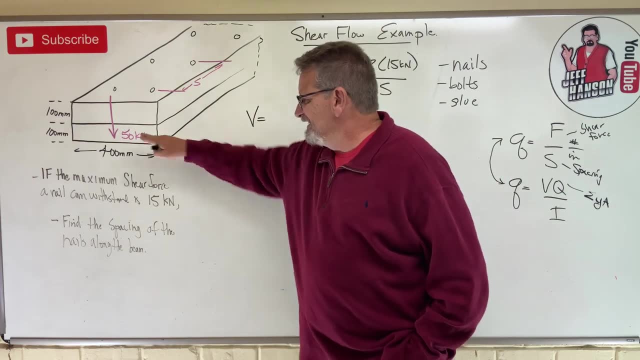 use this equation to find q. okay, So let's do our vq over i. okay, So v. Now, in this particular problem, v is given. What if I gave you a loaded beam and asked you what v to use, What would you? 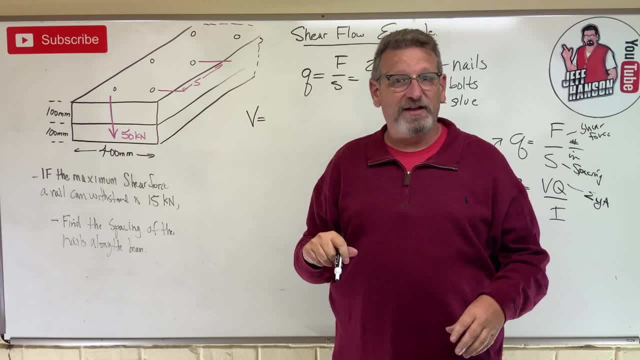 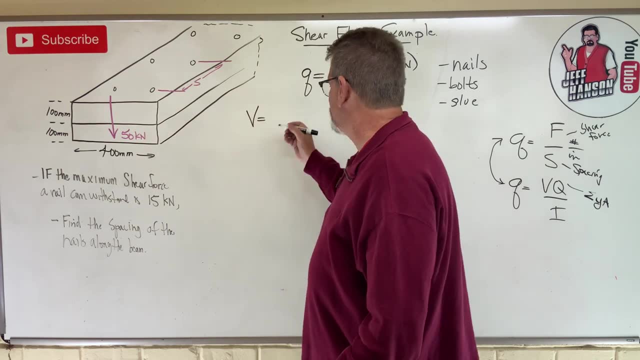 do? I'd just draw a shear moment diagram and find the beam. I'd just draw a shear moment diagram and take its v on the beam and I'd use that v right. But in this particular case they tell us the shear force is 50 kilonewtons, So v is just given 50 kilonewtons. Now again you've got an equation. 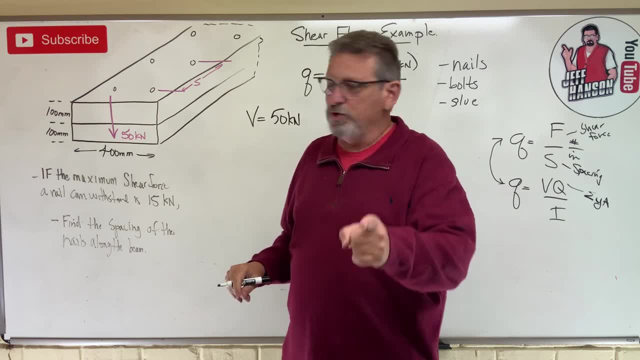 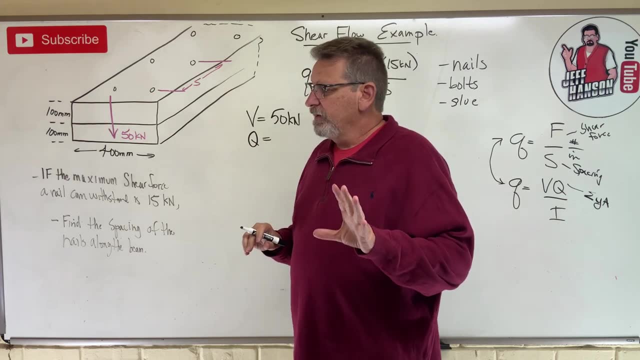 with a bunch of unknowns in it. Make sure to watch your units. okay, Let's see q. what is q Now? the way I like to think about q is: remember. q is the area above or below the point that I'm. 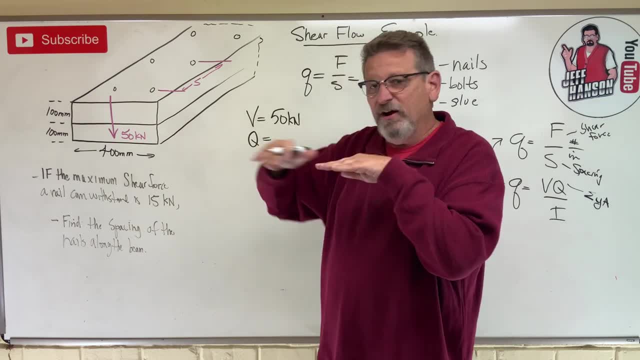 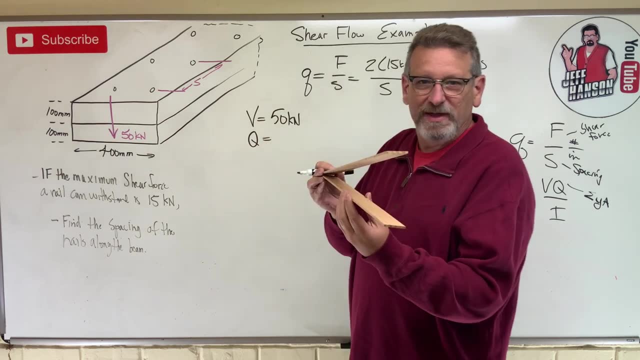 interested in. But I like to think about: I'm going to, I'm going to tear away part of that beam, okay, So if I have something like here's our beam that we have, We have two pieces of wood. they're together right, The nails are in here, But as 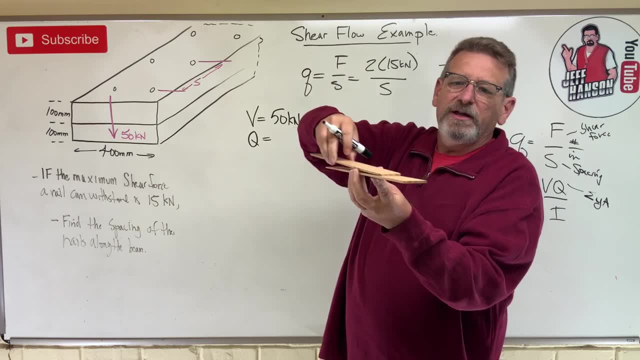 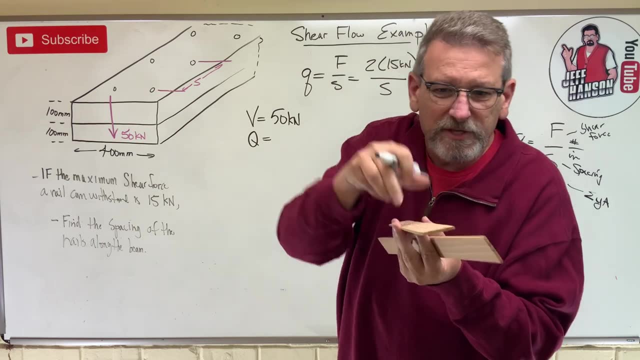 that load is on there, it causes a shear and it's trying to tear this top board away from the bottom board, right. And so what is q, q? is this the area of that board that I am tearing away? Are you with me on that? 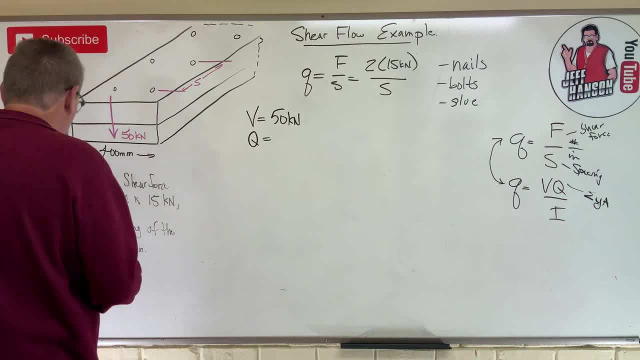 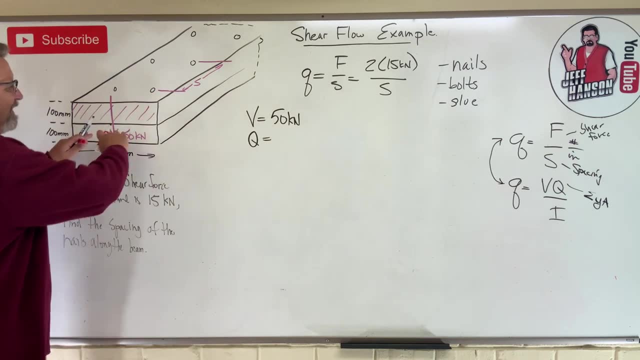 So, on this problem, q is going to be this area right here, Because I'm trying to make this shear plane here fail- where those two boards are nailed together so I can test the strength of those nails and how often do I need to put one. okay, Now I'm going to put a dot here. Why a dot? 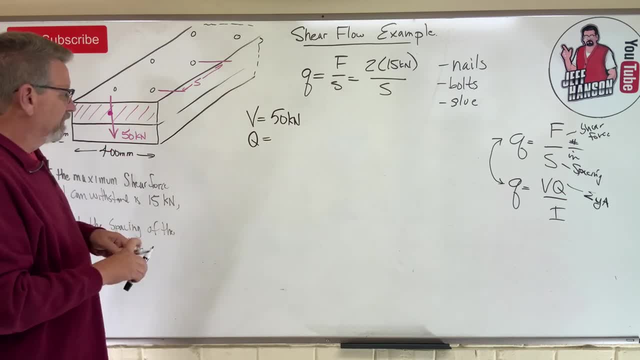 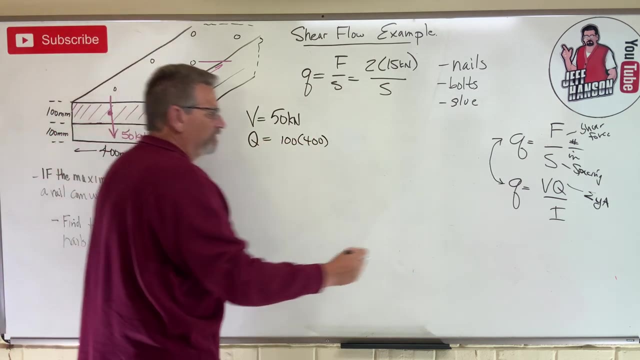 right in the middle of that shape, Because remember, what is q? q is the area above the point of interest. So this plane right here is the one I'm interested in. So q is this area up here which is going to be what? 100 times 400, that's the area. Remember, there's the equation for q, right there, times y. 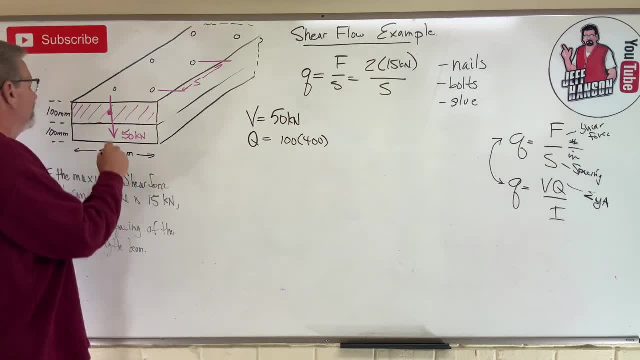 bar, which is always measured from the neutral axis. So y bar, is this distance here? okay, From the neutral axis of the whole beam to the centroid of the piece part? okay, So in this case it's going to be what? 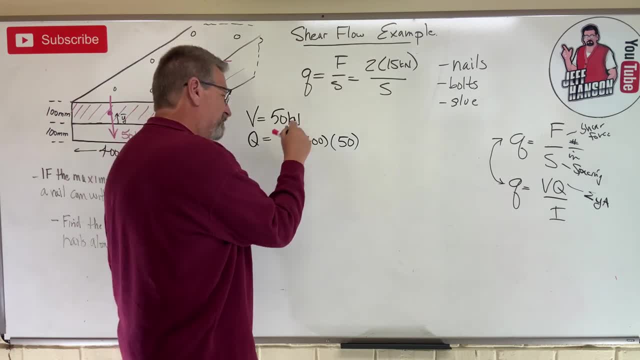 50,. Now again, this is in millimeters, that's in millimeters, that's in millimeters. So Q is going to be in millimeters, cubed, Okay, calculator, what do you got to say to me here? 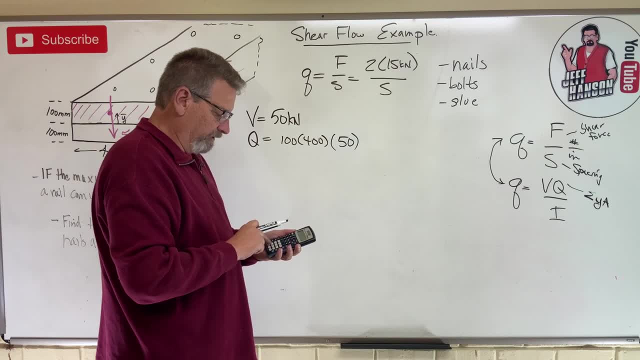 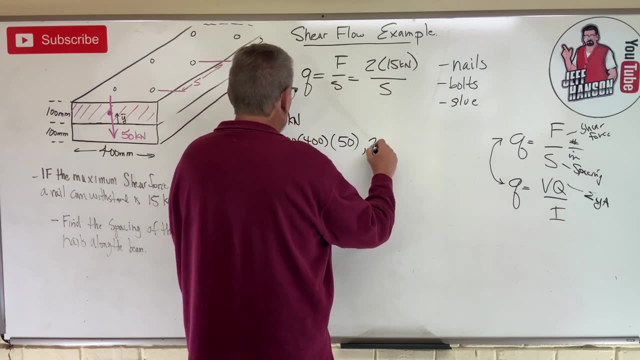 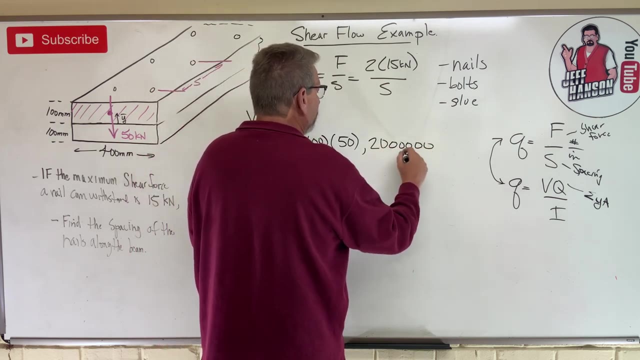 Clear: 100 times 400 times 50 is 2 with a bunch of zeros right: 2, 0 with 1,, 2,, 3,, 4, 5 zeros: 1,, 2,, 3,, 4, 5 zeros. 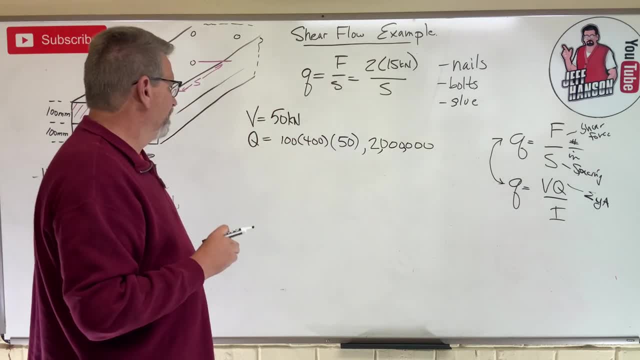 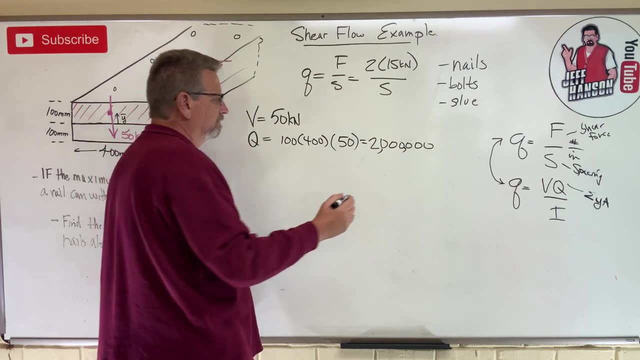 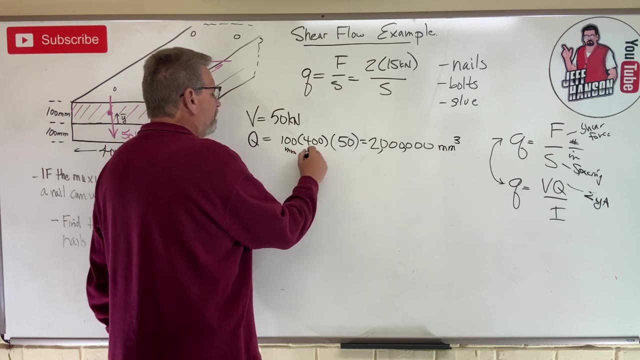 Okay, Okay, 2 million. yeah, that's right, okay, 2 million. and what is the units on that? 2 million, 2 million, what? Well, it's millimeters, cubed right, Because this was millimeters, that was millimeters and that was millimeters. 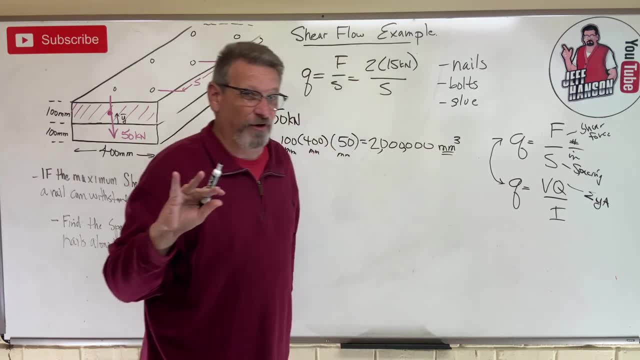 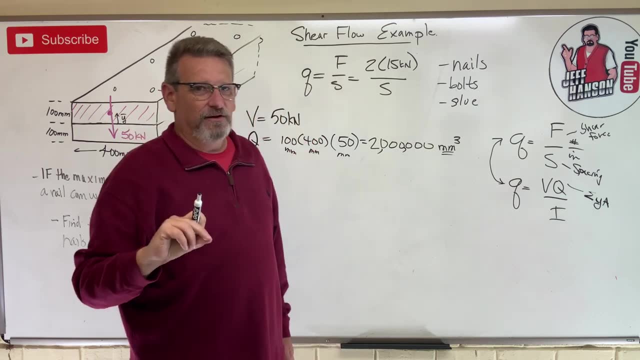 Now remember millimeters, cubed in this case, not a volume. okay, It's a representation of an area and how far away the centroid of that area is From the neutral axis. okay, So it's a geometric property of the cross-section. 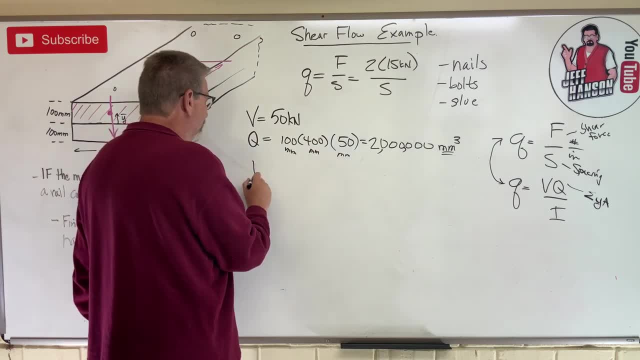 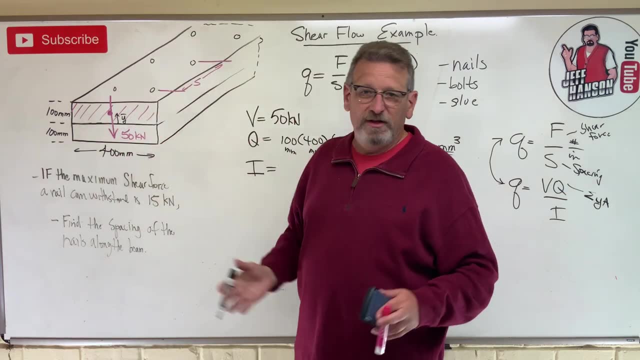 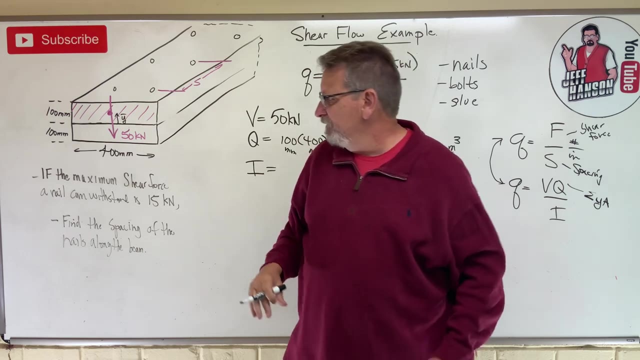 It's not a volume, okay. And then the last thing we need to calculate, little Q is I Now always I on these built-up beams. we still consider the beam, the whole thing, the whole entire beam, both pieces together, to be the beam, okay. 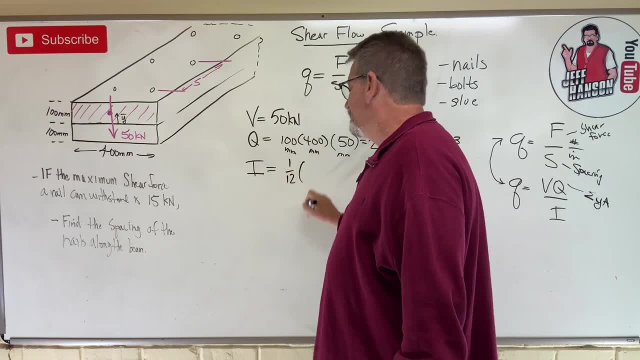 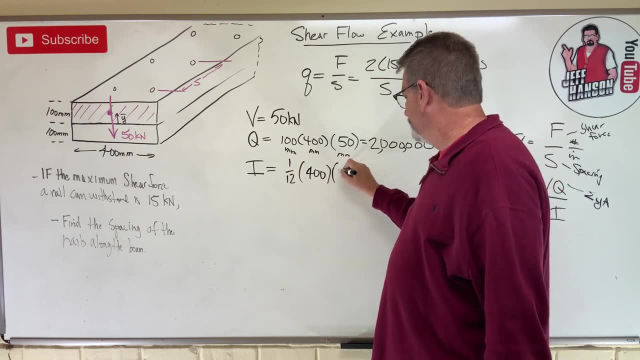 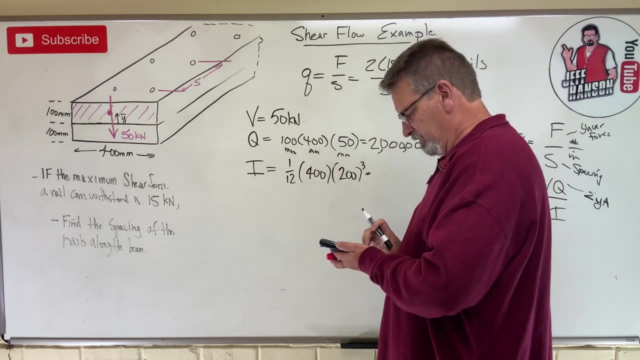 So I in this case, is 1, twelfth the base, which is 400, times the height, which is 200, right, 200 cubed, okay, 2 times 4 is 6.. Oh Lord, what is that number here? 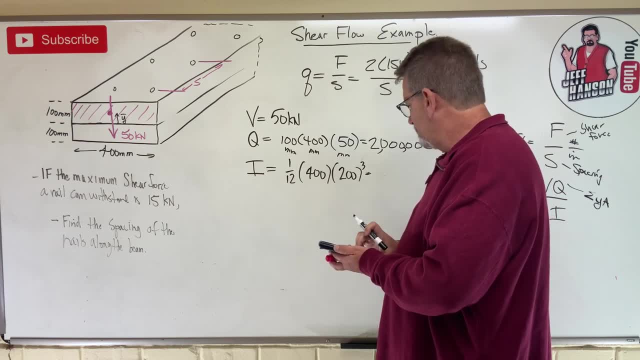 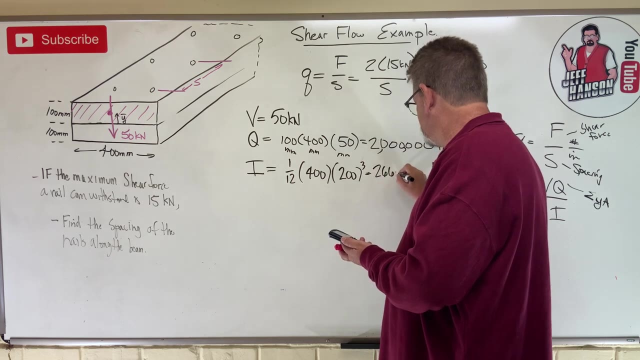 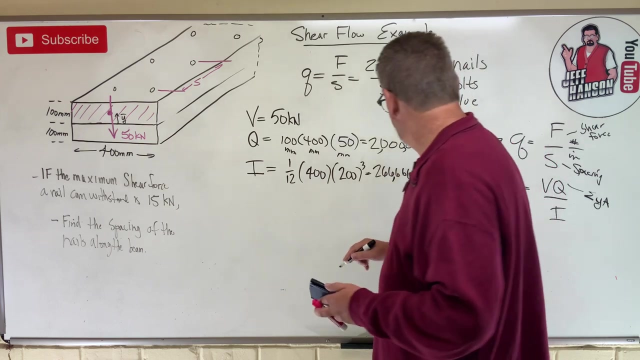 Let's see: 400 times 200, cubed is big number divided by 12 equals okay, 1,, 2,, 6,, 6,, 6,. how many sixes? 1,, 2,, 3, 4, 5, 6,, ooh, 7, 8,. 1,, 2,, 3,, 4, 5, 1, 2, 3, 4,, 5,, 6,, 7,, 8, wah, wah, wah okay. 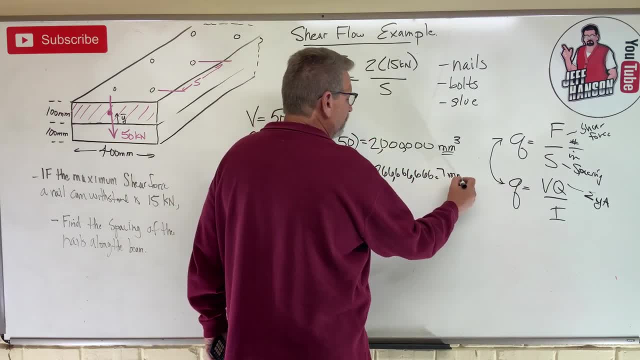 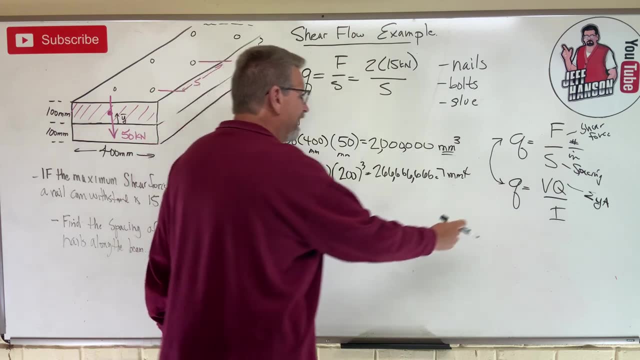 We'll put .7, and what is that going to be? That's millimeters to the fourth. okay, So far, so good. I think we're ready to calculate a little Q here. right, I know that, that and that. 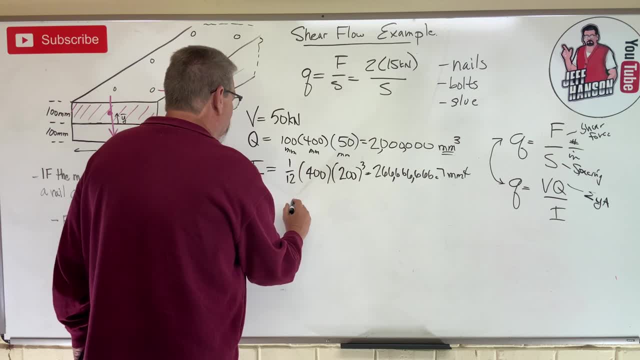 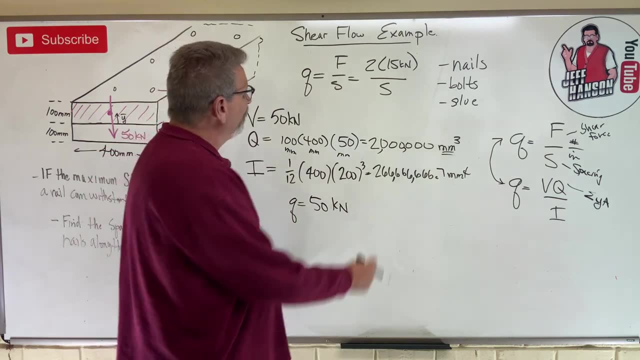 So I can get that guy right. So here we go. Little Q is equal to 50 kilonewtons. Should I convert kilonewtons? You know? no, because little Q up here had kilonewtons. 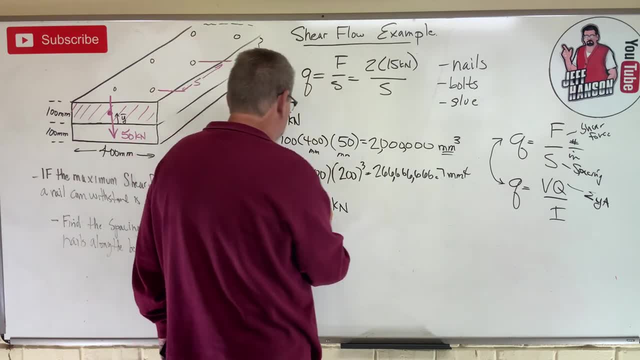 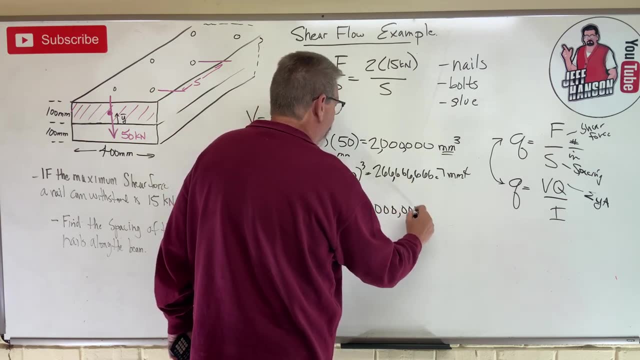 so I'll have kilonewtons on both sides. That's going to cancel out, right. So 50 kilonewtons times little Q, which is 2 million, And of course that is whoop, whoop. a mess is what that is. millimeters Q. 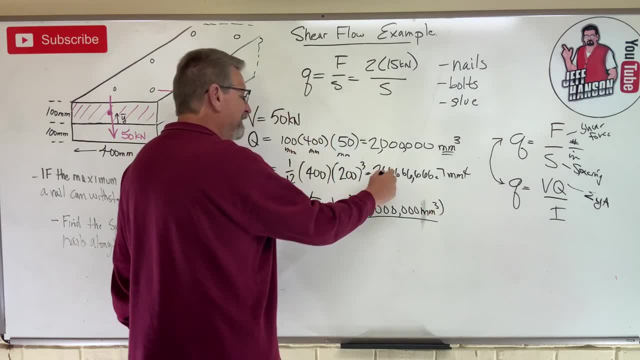 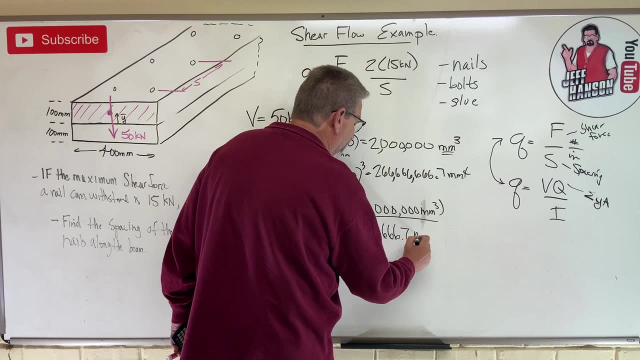 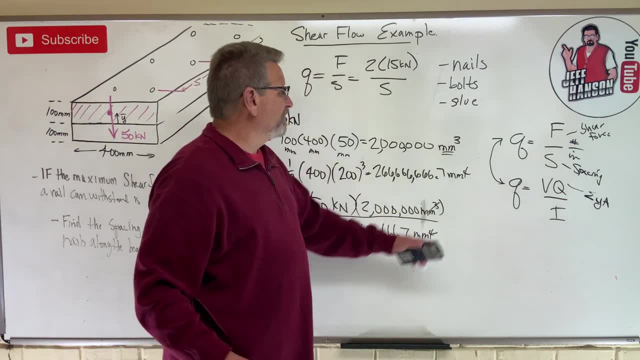 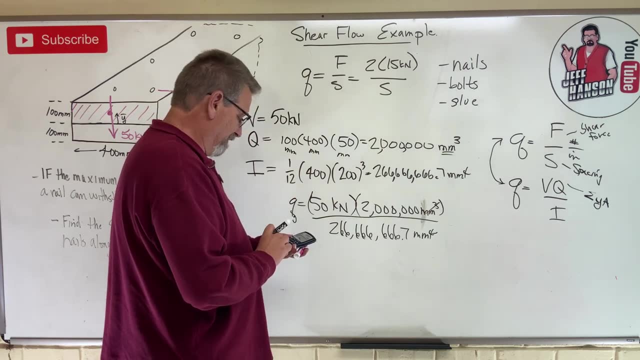 And that's going to leave me with kilonewtons over millimeters, right, Which is a force over length, which is what we want, isn't it? Okay, how much is that? Oh, my goodness, That's 50 times 2 million. 1, 2, 3..